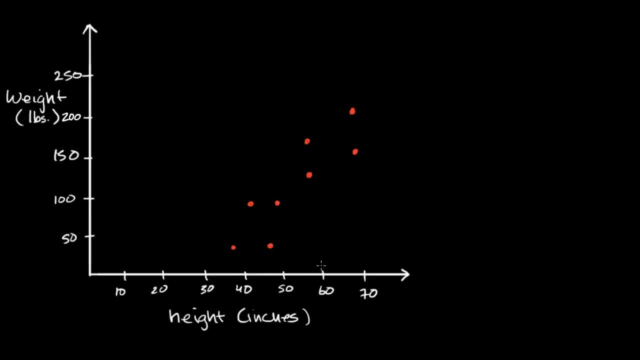 So, for example, let's say I measure someone who is 60 inches tall- that would be five feet tall, and they weigh 100 pounds, And so I'd go to 60 inches and then 100 pounds right over there. so that point right over there. 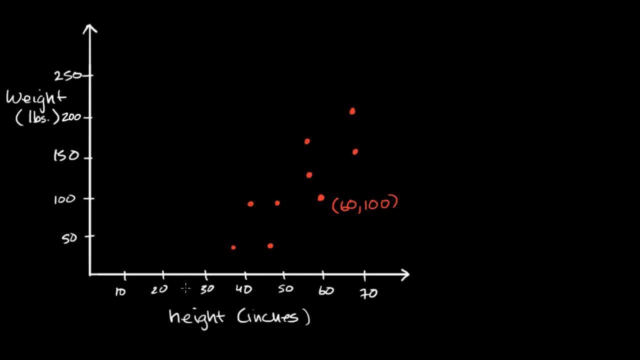 is the point 60 comma. 60 comma 100.. One way to think about it: height, we could say, is being measured on our x-axis, or plotted along our x-axis, and then weight along our y-axis. And so this point from this person. 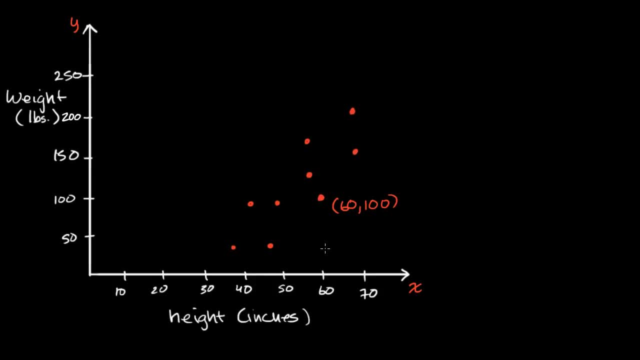 is the point 60 comma 100, representing 60 inches 100 pounds. And so so far I've done it for one, two, three, four, five, six, seven, eight, nine people, And I could keep going. but even with this, 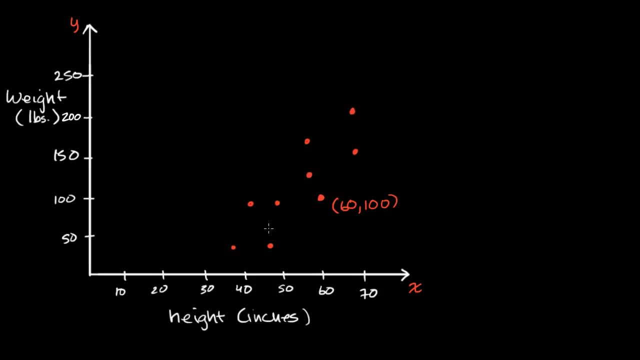 I could say: well, look, it looks like there's a roughly linear relationship here. It looks like it's positive that, generally speaking, as height increases, so does weight. Maybe I could try to put a line that can approximate this trend. 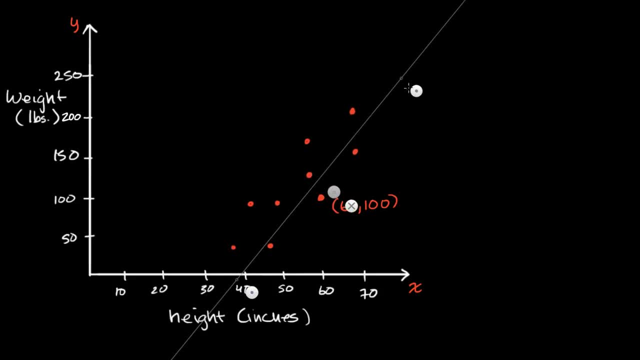 So let me try to do that. So this is my line tool. I could think about a bunch of lines. Something like this seems like it would be you'd be. most of the data is below the line, so that seems like it's not right. 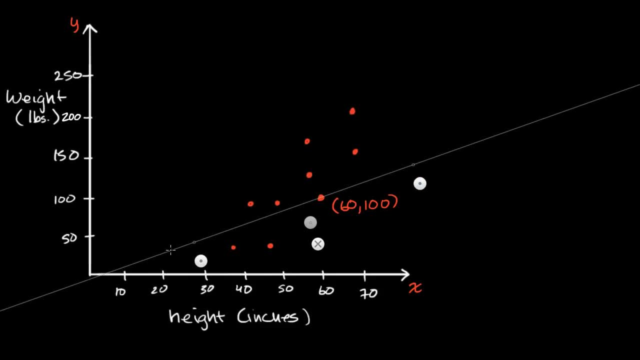 Maybe I could do something like I could do something like this, but that doesn't seem like a good fit. Most of the data seems to be above the line, And so- and once again, I'm just eyeballing it here- In the future, you will learn better methods. 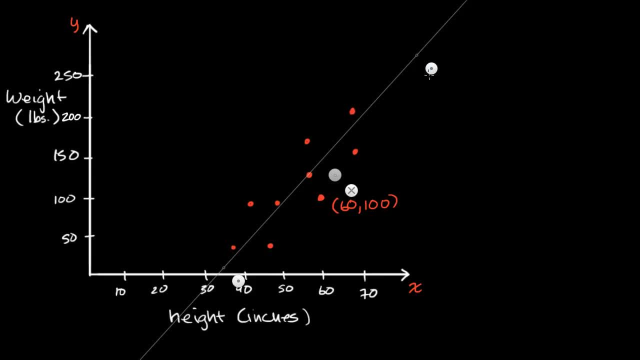 of finding a better fit. but this, something like this- and I'm just eyeballing- it looks about right. So that line, you could view this as a regression line. We could view this as y equals mx plus b, where we would have to figure out. 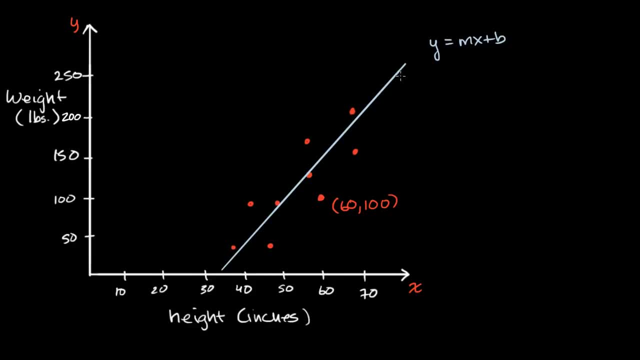 the slope and the y-intercept and we could figure it out based on what I just drew, Or we could even think of this as weight: Weight is equal to our slope times, height times, height plus whatever our y-intercept is, or you could think of it. 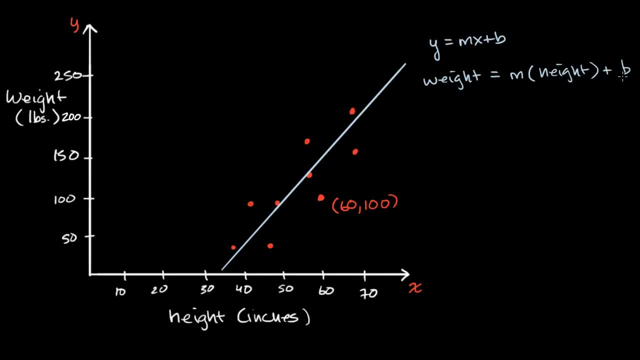 if you think of the vertical axis as the weight axis, you could think of it as your weight intercept. But either way, this is the model that I'm just through eyeballing. this is my regression line. This is something that I'm trying to fit to these points. 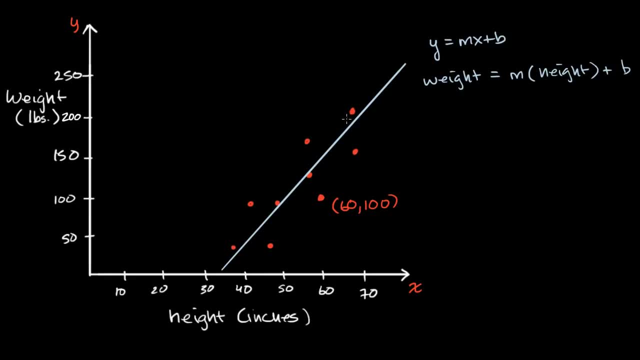 But clearly it can't go through. one line won't be able to go through all of these points. There is going to be, for each point, some difference- well, not for all of them, but for many of them- some difference between the actual 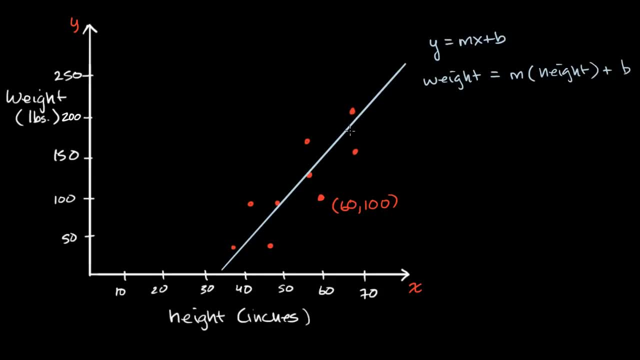 and what would have been predicted by the line And that idea. the difference between the actual four-point and what would have been predicted, given, say, the height, that is called a residual. Let me write that down: The a residual For each of these data points. 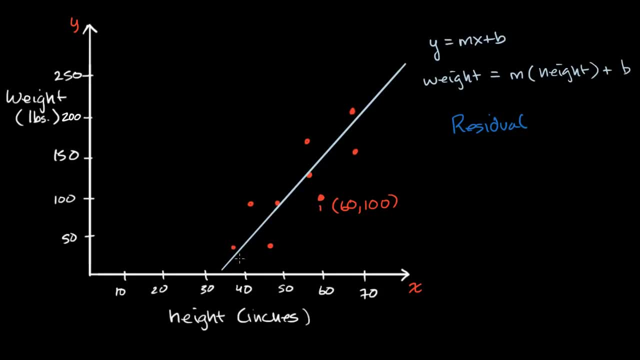 And so, for example, if I call this right here, if I call that point one, the residual for point one is going to be well, for our variable, for our height variable, 60 inches, the actual here is 100 pounds. 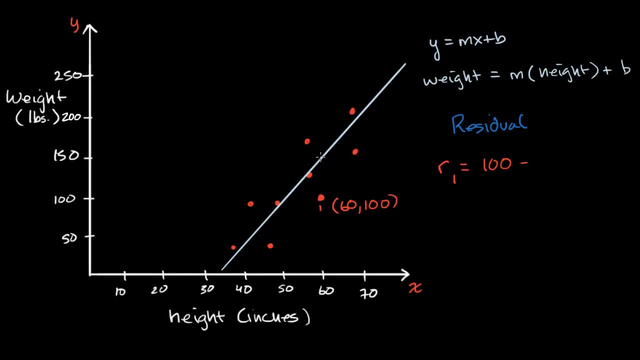 And from that we would subtract what would be predicted. And so what would be predicted is right over here. I could- just I could- substitute 60 into this equation, So it would be m times 60 plus b. So I could write it as: 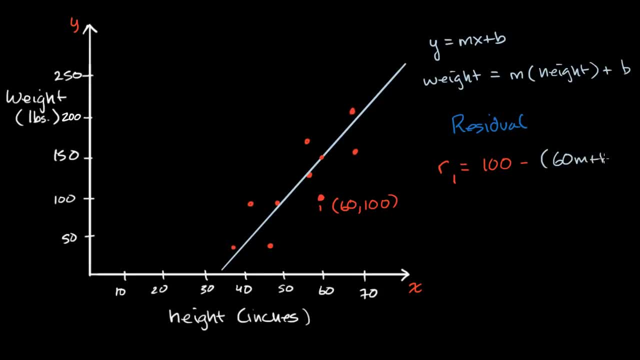 m. maybe let me write it this way- 60m plus b. Once again, I would just take the 60 pounds and put it into my model here and say: well, what weight would that have predicted? And I could even, just for the sake of having a number here. 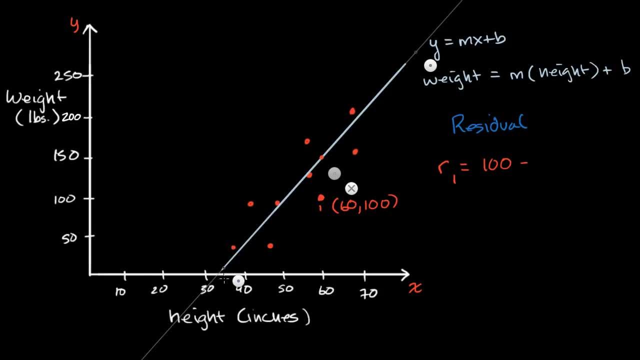 I can look, I can, let me get my line tool out and try to get a straight line from that point. So from this point, From this point, straight, let me get a straight line. So that doesn't look quite straight. 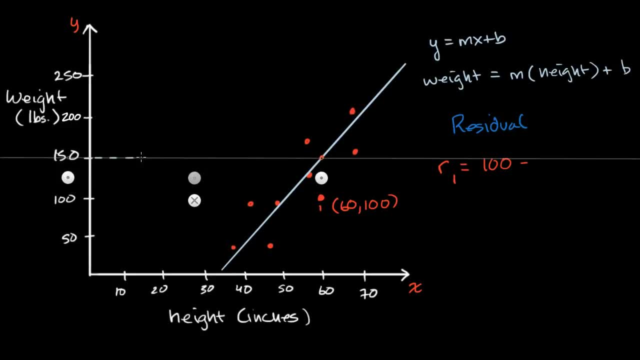 Okay, a little bit okay. So if I, it looks like it's about 150 pounds, So my model would have predicted 150 pounds. So the residual here is going to be equal to negative 50. And so a negative residual is when your actual 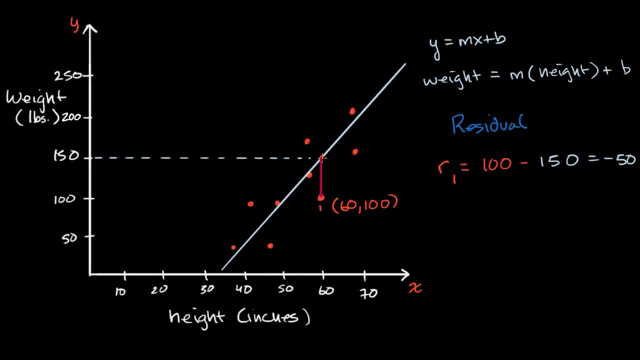 is below your predicted. So this right over here, this is R1. It is a negative residual. If you had, if you tried to find, let's say, this residual right over here for this point, this R2,, this would be a positive residual. 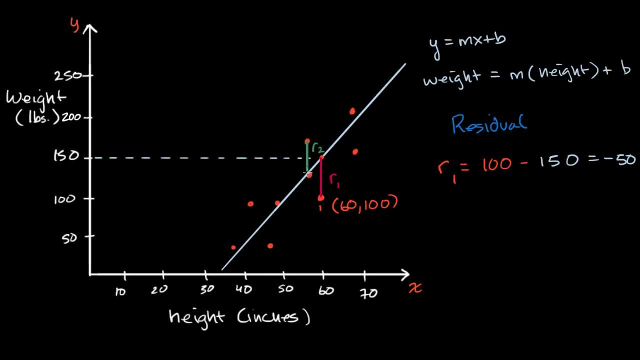 because the actual is larger than what would have actually been predicted, And so a residual is good for seeing. well, how good does your line? does your regression, does your model fit a given data point, or how does a given data point compare to that? 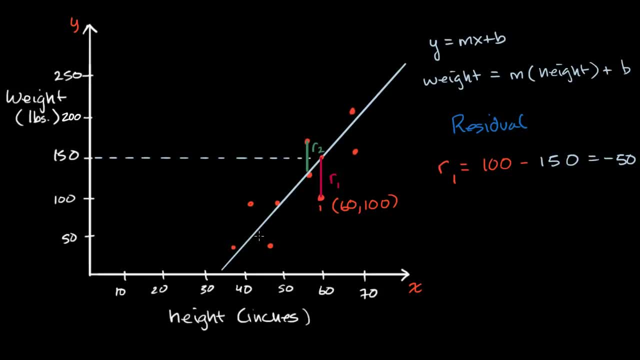 But what you probably wanna do is think about some combination of all the residuals and try to minimize it. Now you might say, well, why don't I just add up all the residuals and try to minimize that? But that gets tricky because some are positive. 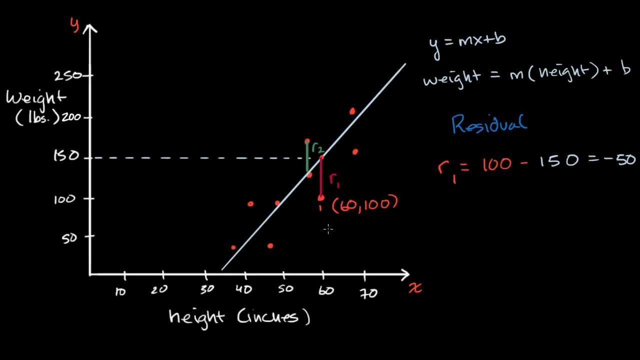 and some are negative, And so a big negative residual- negative residual- could counterbalance a big positive residual and it would look they would add up to zero and then it would look like there's no residual. So you could just add up to zero. 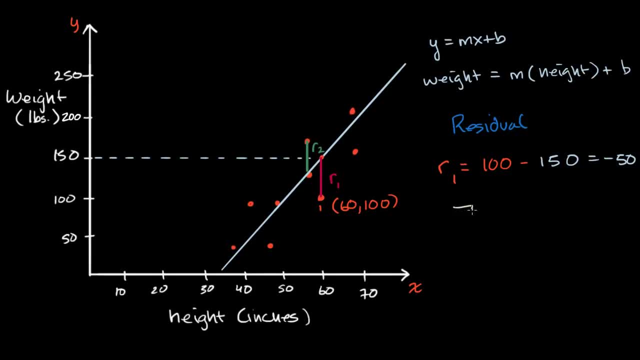 You could just add up the absolute values. So you could say: well, let me just take the sum of all of the residual, of the absolute value of all of the residuals, and then let me change M and B for my line to minimize this. 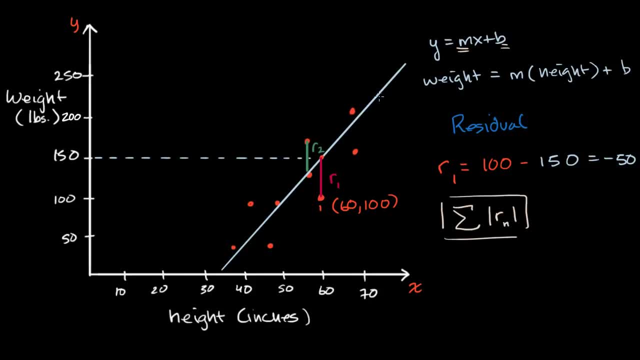 And that would be a technique of trying to create a regression line. But another way to do it- and this is actually the most typical way that you will see in statistics- is that people take the sum of the squares and the sum of the residuals. 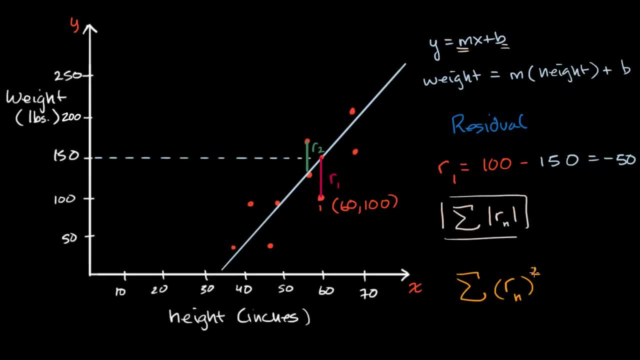 The sum of the squares. And when you square something, whether it's negative or positive, it's going to be a positive. So it takes care of that issue of negatives and positives canceling out with each other. And when you square a number, 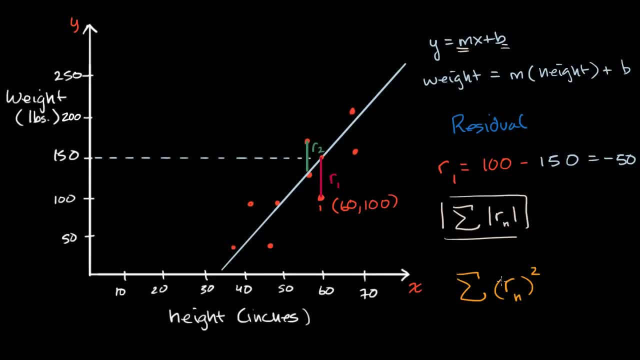 things with large residuals are gonna become even larger, relatively speaking, If you square a large one is. if you think about it this way. let me put regular numbers one, two, three, four. These are all one apart from each other. 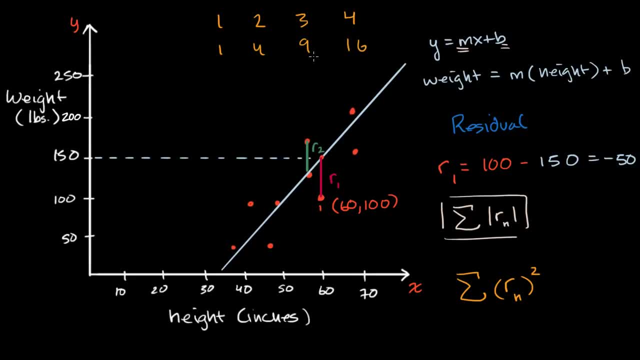 But if I were to square them, one, four, nine, 16, they get further and further apart And so something the larger the residual is when you square it, when the sum of squares, it's gonna represent a bigger proportion of the sum. 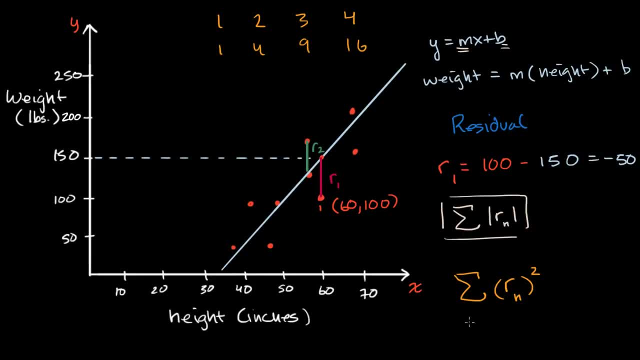 And so what we'll see in future videos is that there's a technique called least squares regression- least squares regression, where you can find an M and a B for a given set of data, and it minimizes the sum of the squares of the residual.